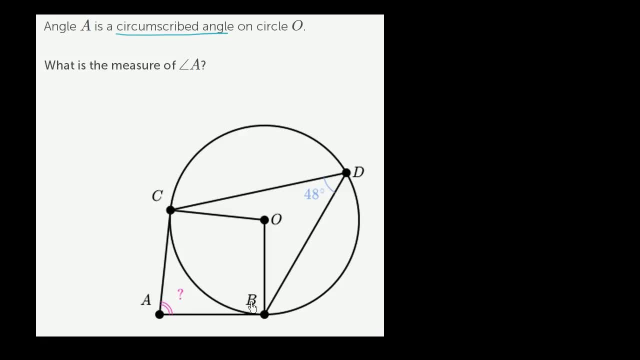 AB is tangent to the circle at point B. What is the measure of angle A? Now, I encourage you to pause the video now and to try this out on your own. And I'll give you a hint: It will leverage the fact that this is a circumscribed angle. 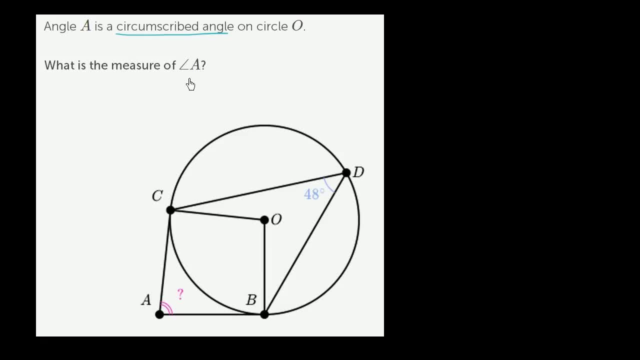 as you could imagine. So I'm assuming you've given a go at it. So the other piece of information they give us is that angle D, which is an inscribed angle, is 48 degrees And it intercepts the same arc. 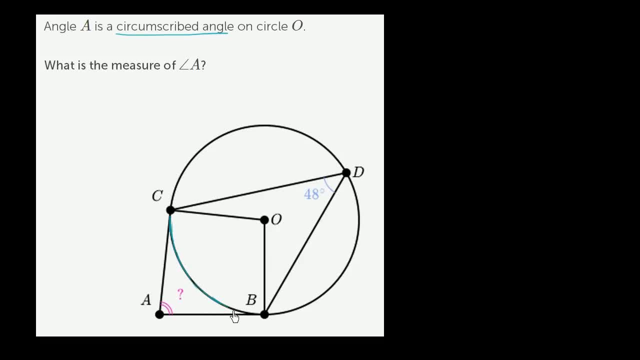 So this is the arc CB, I guess you could call it. It intercepts this arc right over here. It's the inscribed angle. The central angle. The angle that intersects that same arc is going to be twice the inscribed angle. 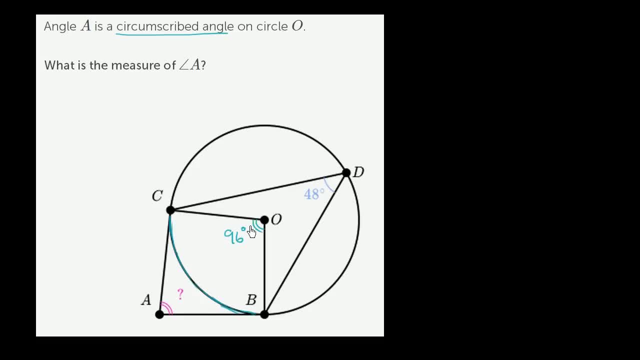 So this is going to be 96 degrees. I could put three markers here. just because we've already used a double marker, Notice they both intercept arc CB. So some people would say the measure of arc CB is 96 degrees. The central angle is 96 degrees. 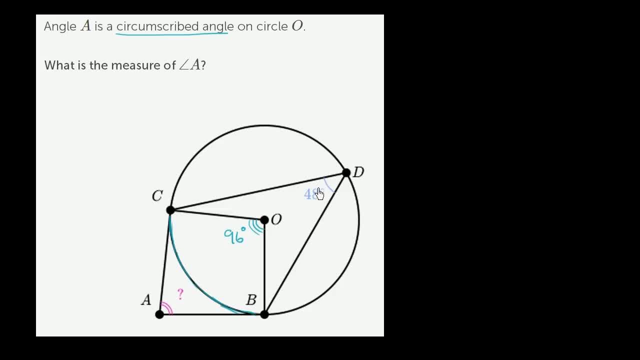 The inscribed angle is going to be half of that, 48 degrees. So how does this help us? Well, a key clue is that angle is a circumscribed angle, So that means AC and AB are each tangent to the circle. 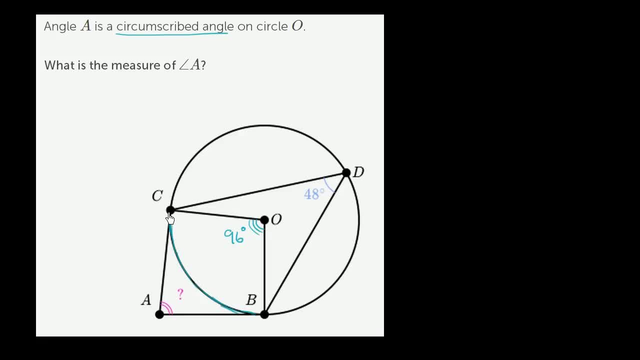 Well, a line that is tangent to the circle is going to be perpendicular to the radius of the circle that intersects the circle at the same point. So this right over here is going to be a 90 degree angle And this right over here is going to be a 90 degree angle. 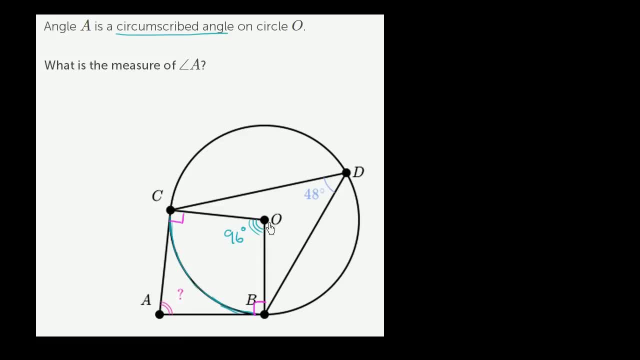 OC is perpendicular to CA, OB, which is a radius, is perpendicular to CA, And this is perpendicular to BA, which is a tangent line, And they both intersect right over here at B. Now this might jump out at you. We have a quadrilateral going on here.